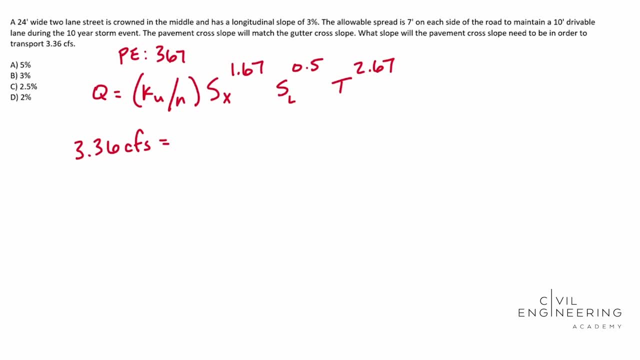 Alright, and our KU is actually given as 0.56.. That's given to us on that page, 0.56.. Divide that by N, Which is our roughness coefficient. You can find that on page 388.. We will get 0.011.. 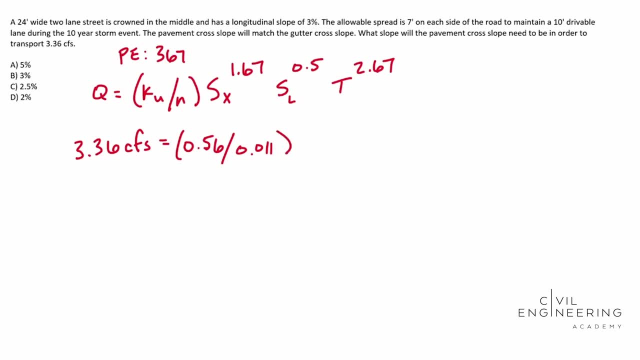 That's a good, safe number. And then we have SX, which we are solving for the cross slope to the 1.67 power. And then we have SL, which is our longitudinal slope. It gives it to us in our problem it's 3%, so 0.03.. 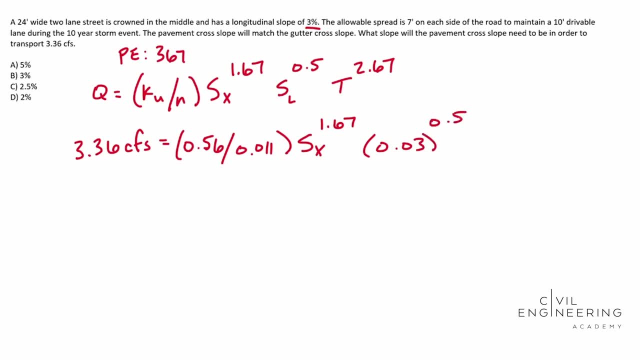 Make sure it's written in decimal form. This is to the 0.5 power. Then we have our spread. So this is our allowable spread. What we are calculating is one side of the road. If you're going to kind of picture a road that's crowned in the middle, it's a two lane. 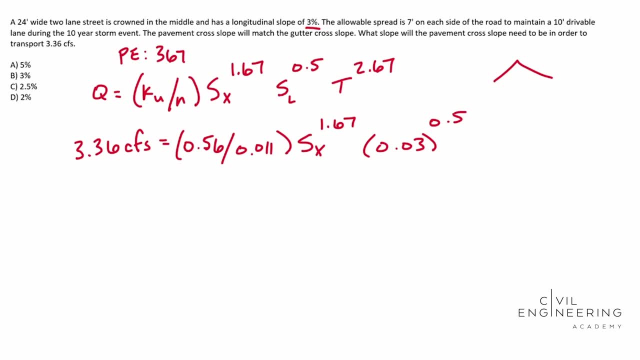 So we know there's one lane on each side. that's 12 feet. It says our allowable spread is 7 feet, So you can kind of picture if you have an inlet right here collecting. we can't have water more than 7 feet into our road. basically. 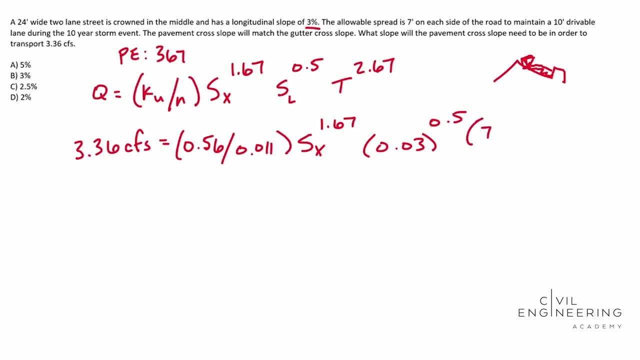 So this is that's our maximum. so our spread is going to be 7 feet. So 7 feet and we're going to raise that to the 2.67 power. So really, you'll notice that we only have one unknown here. 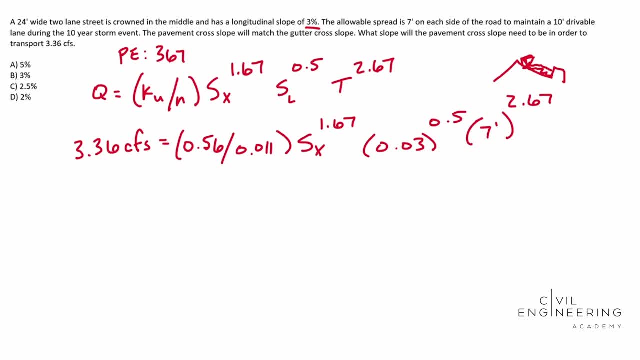 And all we have to do is solve for SX. Okay. so now all we have to do is simplify. So 3.36 cubic feet per second And we're going to put that over our 0.56.. Over 0.011.. 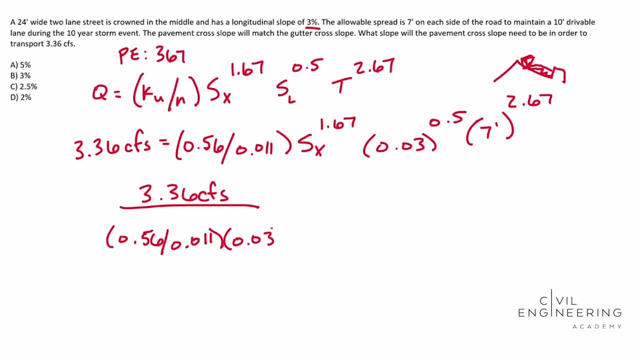 We're also going to bring in the 0.03, raise that to the 0.5.. Multiply that by our 7 foot and we're going to raise that to the 2.67 power, And all of this ends up being equal to the cross slope to the 1.67 power. 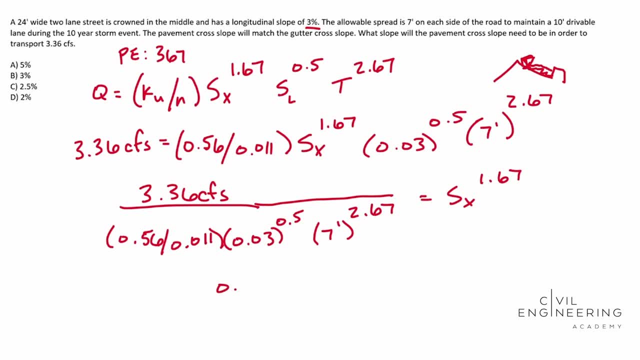 So we're going to multiply that by our 7 foot and we're going to raise that to the 2.67 power. So whenever you simplify this out, you should end up with something similar to: 0.00211 is equal to the cross slope to the 1.67 power.